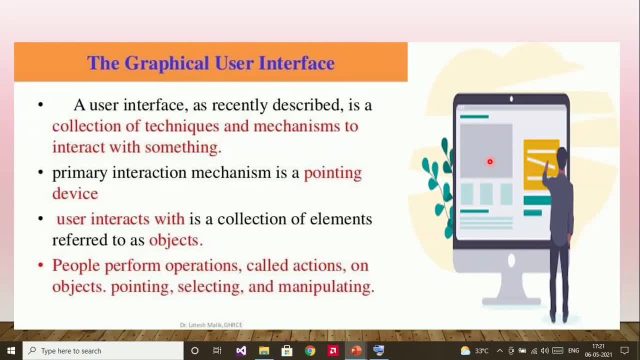 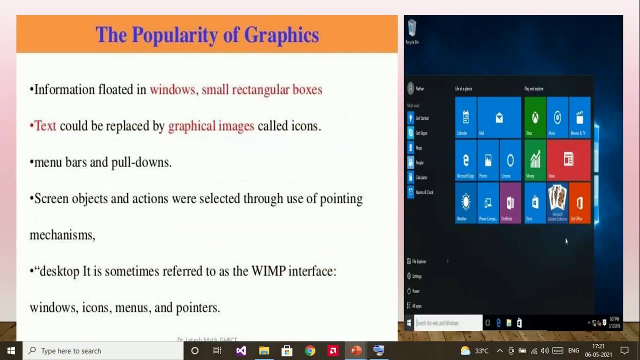 They are independent of all other objects. Okay, people perform operations, called actions, on those objects, and the operations include accessing and modifying objects by pointing, selecting and manipulating. All the objects have standard Resulting behaviors. The popularity of graphics: Graphics actually revolutionized the design and user interface. 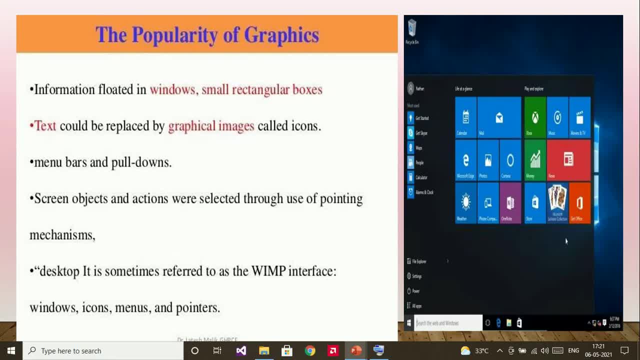 Earlier we had text based user interface, but nowadays all the informations, whatever you have, are going to be floated on Windows using a small rectangular boxes. So, as you see here One of the example, you can see that it is a user interface you have here and the information, whatever you want, is being floated on Windows screen and it's all represented using small rectangular boxes. 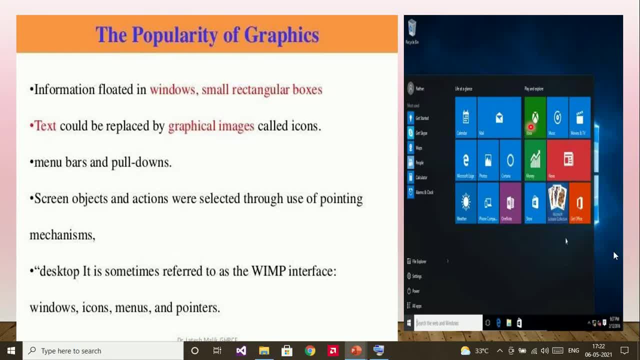 Okay, and text based graphical user interface are replaced by graphical images called icons. So nowadays we all have icons on the screen. We also have menubas and pulldown pulldowns also. screen navigation commands are executed through menubas and pulldowns. 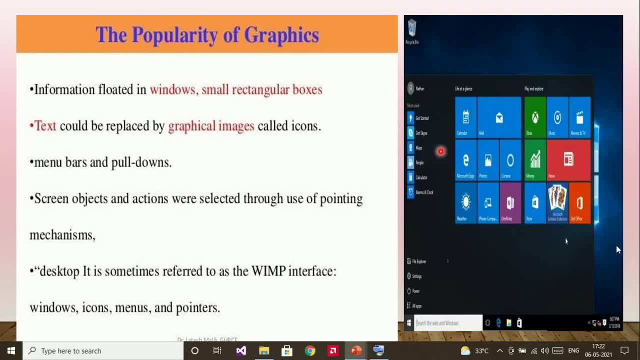 Menus pop up on the screen Okay, and in screen body. the selection fields such as radio buttons, checkboxes, listboxes and palettes are also being used. Screen objects and actions were selected through. objects and actions were selected through some of the pointing uh mechanisms, such as mouse or. 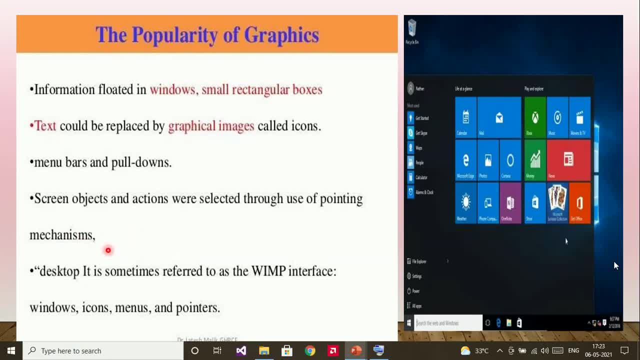 joystick instead of using traditional keyboard. so nowadays we use pointing mechanisms mainly for pointing any object on that is on the screen. okay, we generally use mouse and joystick and the desktop. nowadays, whatever we use, we sometimes refer to as wmp interface. wmp stands for windows icons, menus and pointers. okay, so this wmp stands for mainly windows icons, menus and. 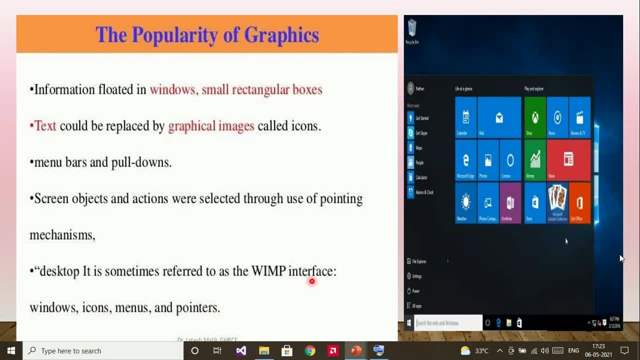 pointers, so now we call it as wmp interface. okay, and uh, the graphics, uh also adds appeal or charm to the interface and it permits customization to create a unique corporate or organization styles, and you nowadays have mainly customized user interfaces are being developed for the customers or organizations. 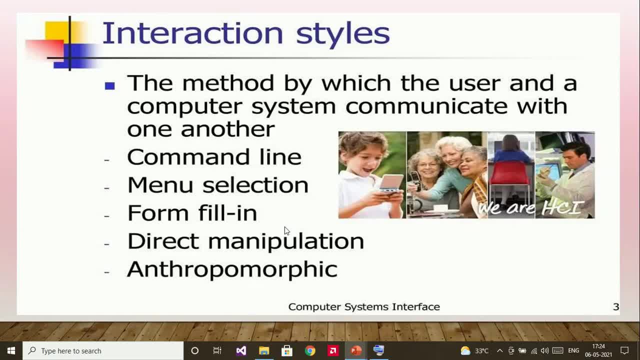 interaction styles. the method by which the user and the computer system communicate with each other is called a interaction style. so now we normally use command line menu selection method, form fill in method, direct manipulation of interaction style. we use- and also sometimes, uh, humans use- anthropomorphic method for interacting with the computer or the system. 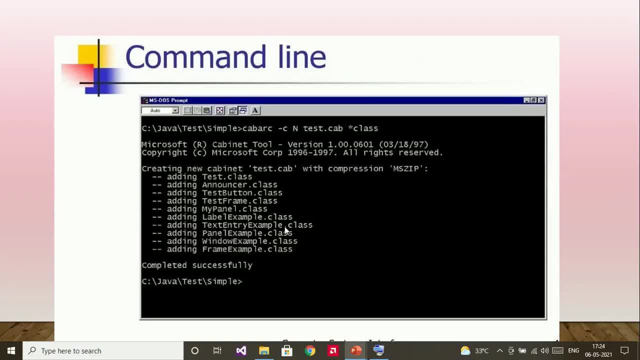 kind of interaction style is command line. so this is an example here to show how the command line interface looks like. okay, everything it has to be written and memorized. okay, the commands has to be memorized before writing anything or typing anything on the screen. and, as you see here, this is msdos prompt and you have a black color background and a simple white text. 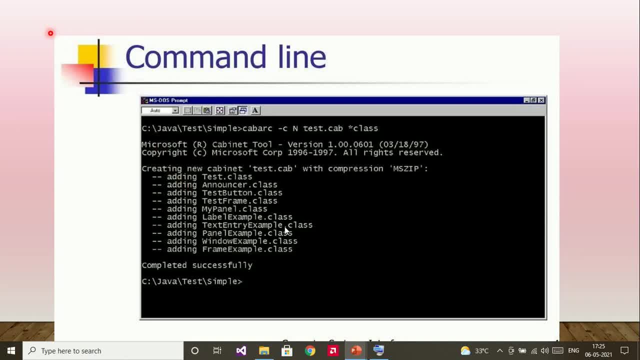 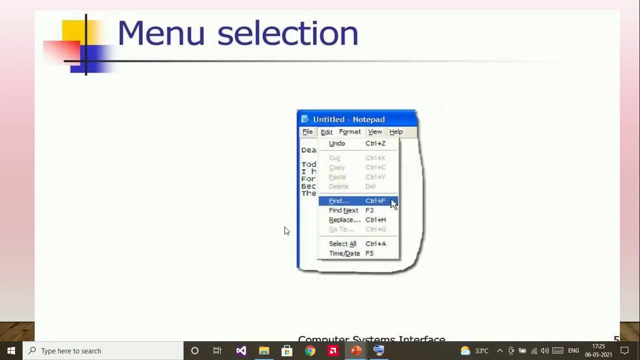 it is okay. so this was earlierly used as the first interaction style that was used by the user to interact with the computer. next kind of interaction style is menu selection method. so, as i said, screen navigation and commands are executed to menu bars and pull downs. so here you can see a pull down menu. 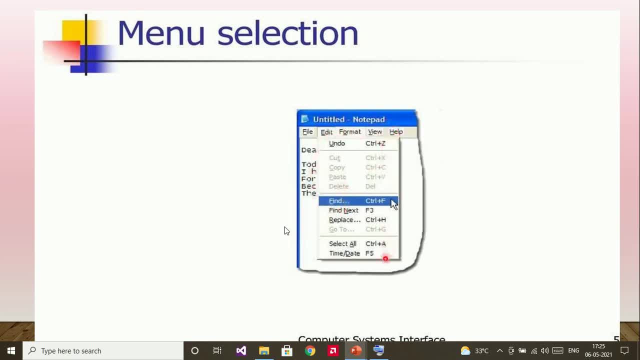 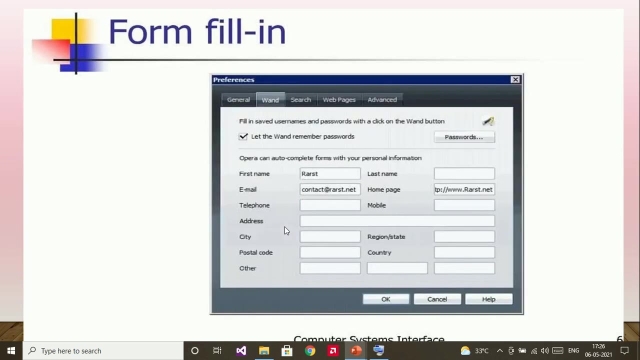 and you may have along with this menu, so you may have check boxes, list boxes, pallets, radio buttons, everything will be used. okay, the next method of interaction style is form fill-ins. so, as you can see here, this is a latest kind of interface we have, where you are using form fill-ins. okay, you may have to fill the names, okay. 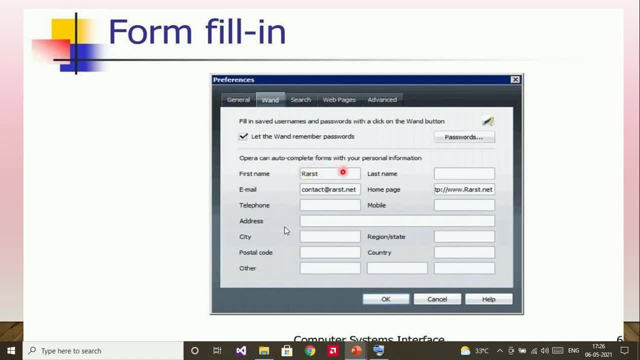 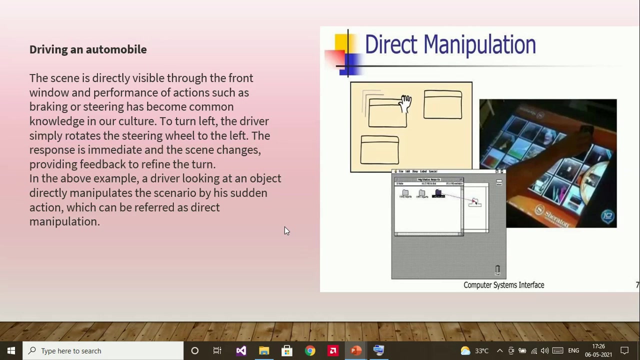 you have to type here certain name- okay, alphabets here- and also along with this you may get pull down menus, check boxes, list boxes, everything in this kind of forms also. next kind of manipulation, uh, or interaction style we have that is direct manipulation, so actually in our user interface. 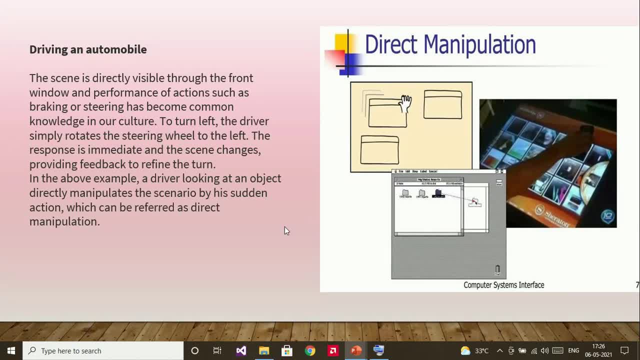 chapter. we have two kinds: direct in direct manipulation and indirect manipulation. so let me tell you how a direct manipulation works. okay, consider: uh, you're driving an automobile and you're seeing that particular scene. uh, how, the how you feel when you're driving the automobile. that scene is directly visible at that scene. okay, right now we're talking about a direct 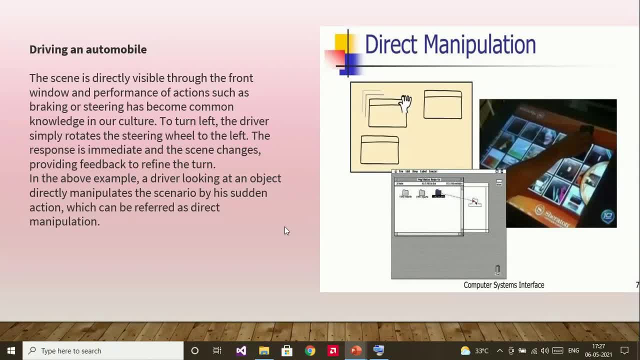 the front window and performance of actions such as breakings and steering is being done everything all feel you will be having to turn left. the driver actually simply rotates the steering wheel to the left and the response will be immediate and the scene changes on this, on the particular screen providing 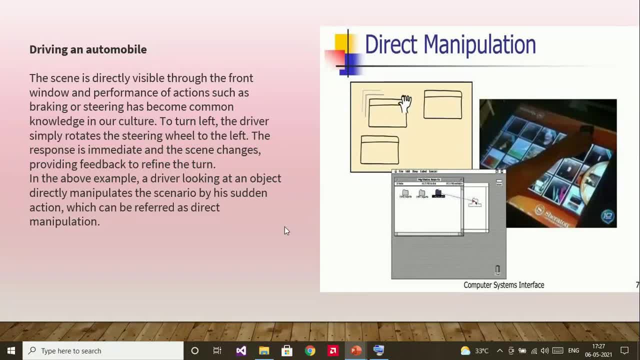 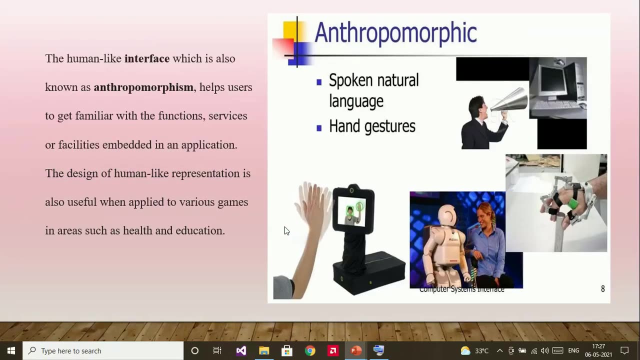 the feedback to the refined to refine the turn. okay. in this particular example, driver looking at an object directly manipulates the scenario by his sudden action. okay, which is referred to as direct manipulation. another kind of interaction style we have that is anthropomorphic interaction. human-like interface, which also is known as anthropomorphic, helps the user to get. 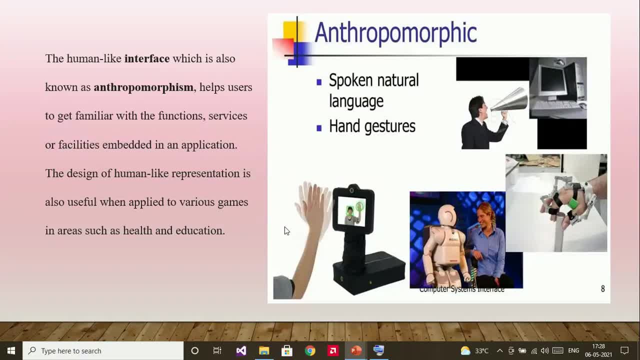 the feedback to the right direction and the feedback to the left direction is familiar with functions, services and facilities embedded in an application. the design of a human-like representation is also useful when applied to various schemes in areas such as health and education. so, as you can see, for example, your out our movie or the lion- the lion movie you have okay. 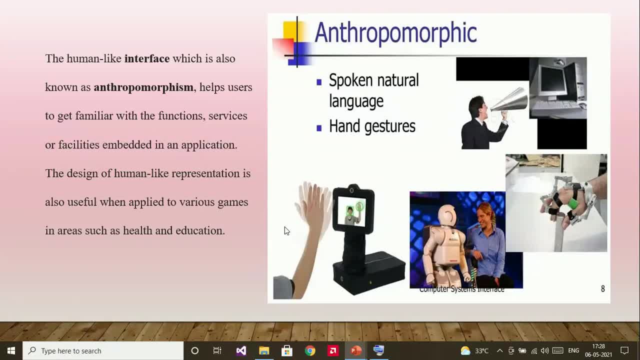 all these were done using anthropomorphic mechanisms. okay, there will be certain gestures, as you can see here, the hand gestures- okay, will be provided to the system. okay, and there will be a certain mechanism to convert that particular image to another kind of image- okay, or video. so there will be direct human to human interaction in this kind. 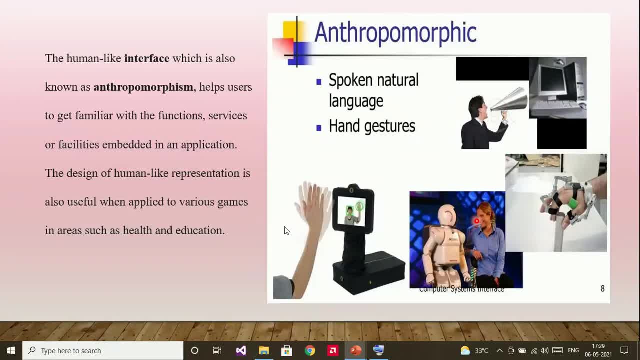 anthropomorphic style of interaction, you may feel like you are interacting with the human itself. okay, so here one more example you have. one girl is speaking to a robot, so this robot responds in such a way that- but it is, it responds like a human itself. so this is based on anthropomorphic mechanism style of. 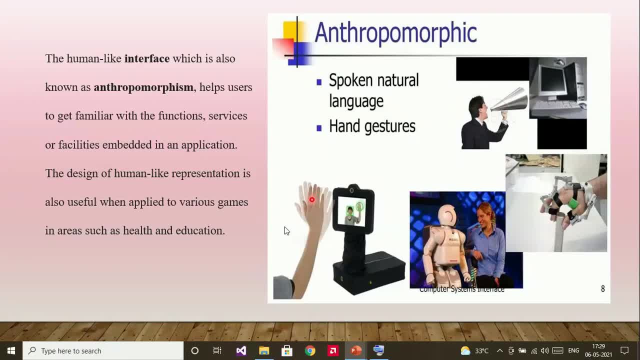 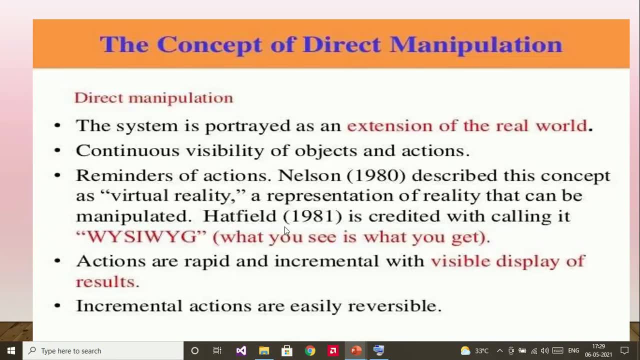 interactions they are using. yeah, next concept is reptilian interaction. you have that is direct manipulation. so this is very important concept here in this particular module. the term used to describe the style of interaction for graphic systems was first used by snail done man in 1982. he called it as direct. 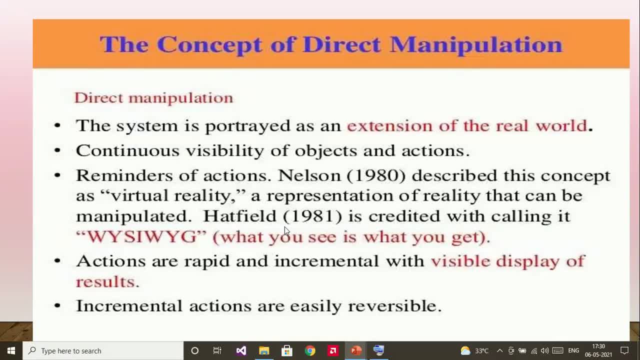 manipulation systems. okay, so the term, actually the direct manipulation, was given by snail done man. okay, so he suggested that in the direct manipulation systems there are few characteristics. so let us see what are the main characteristics here. the first main characteristics is: the system is portrayed as an extension of real world, so it is assumed that the person is. 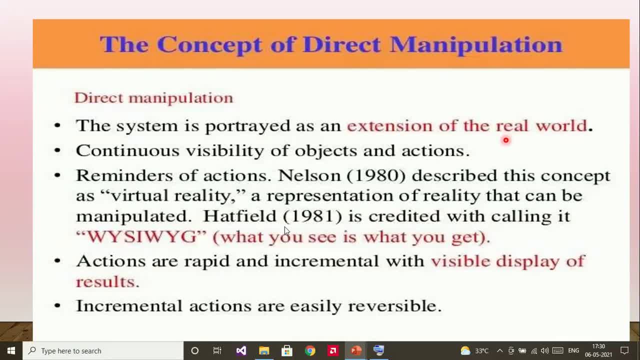 already familiar with the objects and actions in this environment, and then the system is portrayed as an extension of real world. and then the okay, and the system actually replicates them and portrays them on the different medium that is called the screen. okay, so here, actually, the person is already familiar with the objects. 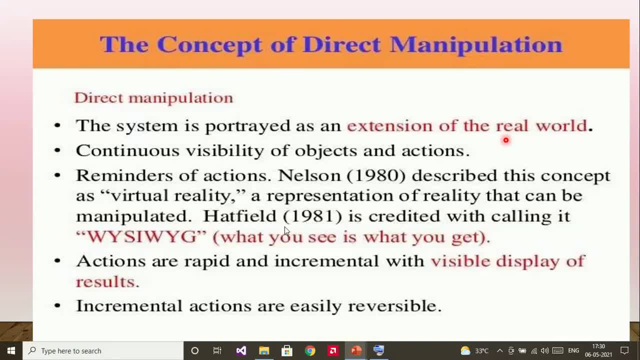 and and what actions he has to do. for example, you say: here you are using a window. okay, you are using a window, you can close it and open it, you can minimize it or you can maximize it. is it so? that is one of the example for direct manipulation, or something you, some file you have? 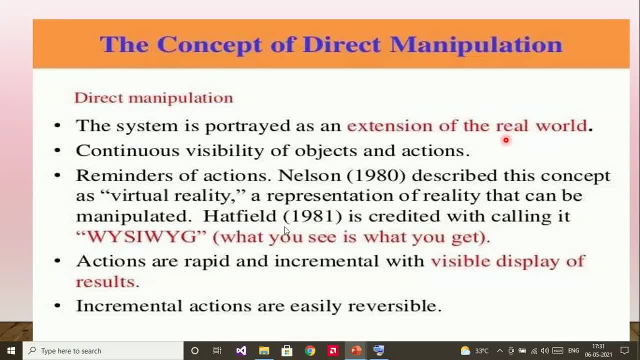 outside the window, you drag it and you keep it on the exact location inside the window- okay, window of the screen. so that is also. dragging of a file is also a direct manipulation. you can say, or something like that: so that is one of the example for direct manipulation. 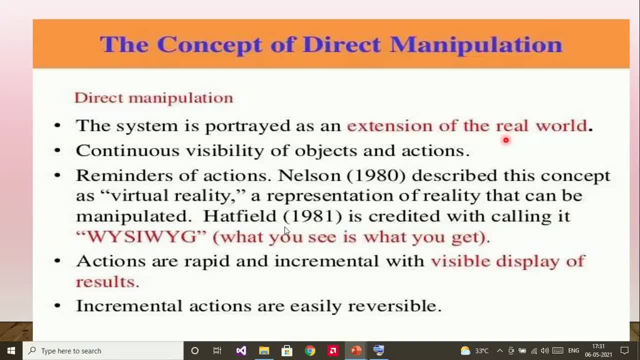 times you use gaming, gaming tools, where you are using a keyboard or mouse for directly manipulating the objects which are present on the screens. okay, so here the it is assumed that the person is already familiar with the objects and actions, what he has to do with the environment. 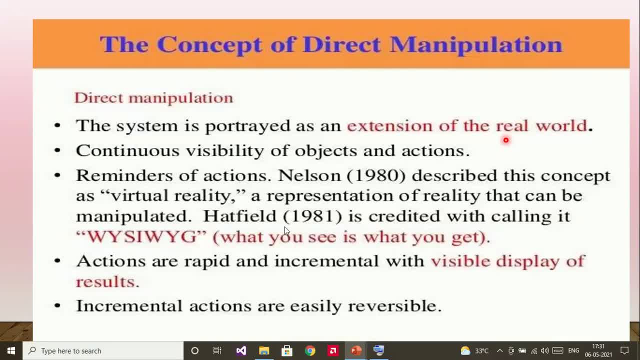 and the system simply portrays that on the medium- okay, and here the person has the power to access and modify the objects on the screen. okay, or on the whatever it is displaying on the window. hmm, so here this is one of the first main characteristics: any direct manipulating. 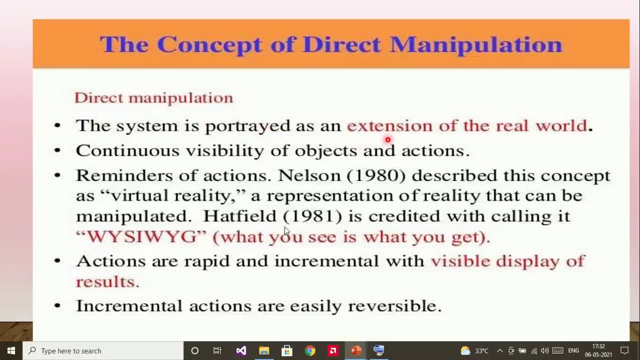 system should have. the system should is portrayed as a system which is able to as an extension of real world. okay, and other example you can give it, as if you are using a pdf, you might have used zoom, zoom in and zoom out operation. so this, this operation, is already. 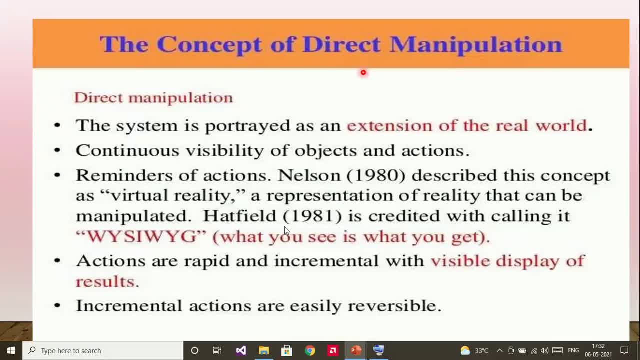 you are familiar. okay, no need of training you with that kind of action. okay, so you are familiar. the person who are who are using the system is already familiar with the objects and actions in his environment. so here, the person who is using the system is already familiar with the objects and actions. 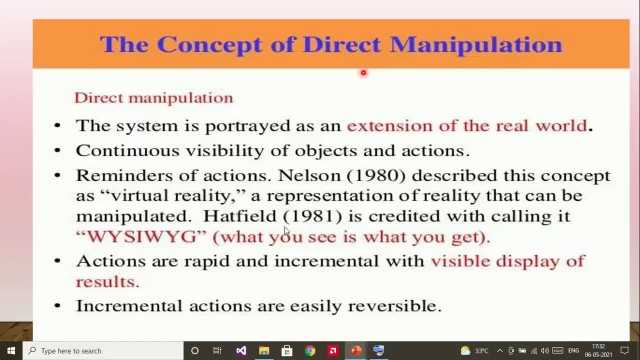 and the system actually portrays that as a extension of real world. next one is. second point is continuous visibility of objects and actions. so here the reminders of actions that are to be performed are already labeled using buttons. okay, now we have labeled buttons. before they were using syntaxes and command names. but 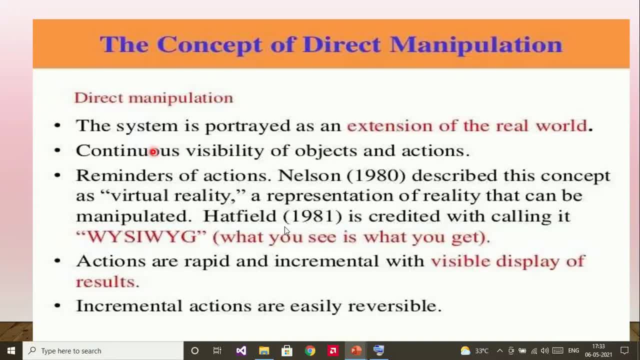 now, nowadays we have labeled buttons for any interactions with the computer. okay, so, uh, nelson. in 1980 one person called nelson. he described this concept as virtual reality. so that is my direct manipulation concept as a virtual reality. so this was given by the person nelson, and 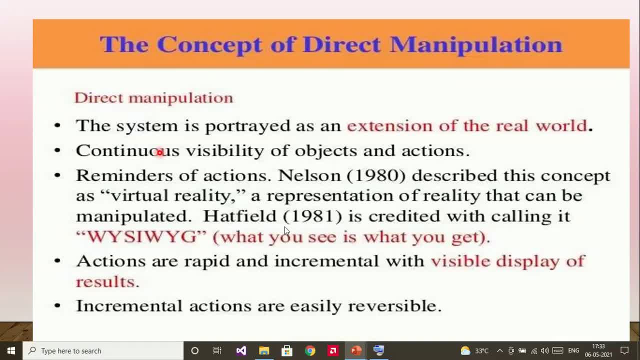 actually why he has given that particular name is The system was representing the reality that can be manipulated. And next person in 1981 called Hatfield. He described it as visigwig, Named it as visigwig. Okay, What you see is what you get. Another person has named it as this kind: What you see is what you get. And some other person, Holland and Norman, in 1986. they considered direct involvement with the world of objects rather than communicating with the intermediaries. 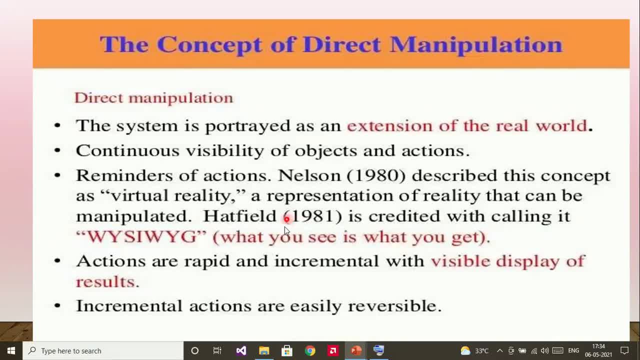 Okay. So actually the thing is here. what you have to explain here is continuous visibility of objects. So continuous visibility of objects and actions means: suppose in the real world what you have. For example, you have a paper. Okay, The paper size cannot be manipulated, Is it? It never shrinks or it never grows, It is of a constant size. But the same kind of paper can be manipulated in the system. Okay, You may add more content to this. 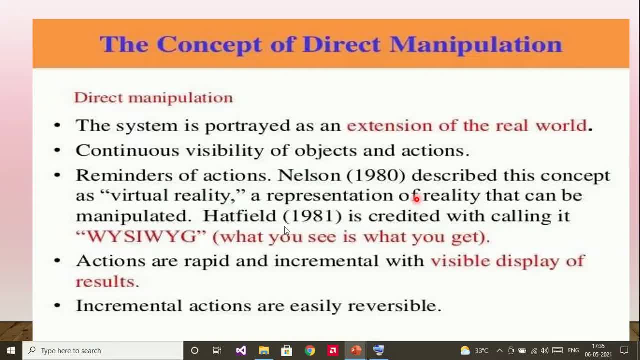 You may add more content to the screen or the page, Is it? And then you can manipulate any contents. whatever is there in the window system, Okay So. or similarly, you can say: a window which has got a border can also be manipulated in using your mouse or your any system you are using. Is it The window border? Whatever you have created, Maybe also it can be manipulated. 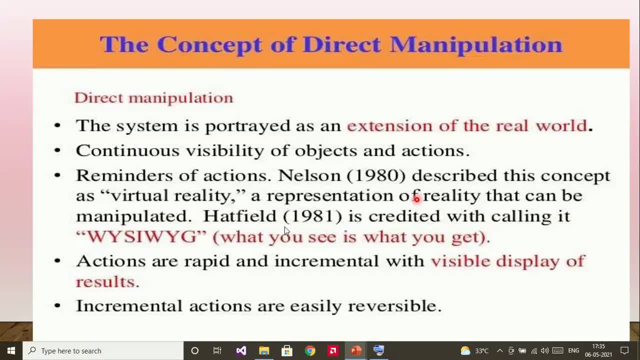 Can be also manipulated. The control panel can also be manipulated. So there are many different examples, which which are the things you can manipulate in your screen. So actions. Next point is. fourth point is: actions are rapid and incremental, with visible display of results. 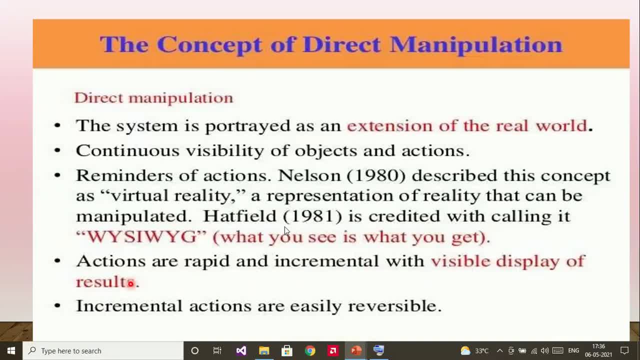 Okay, So actions are rapid and incremental, with visible display of results, Since the touch Feedback is not actually possible in the existing user interface, but the screen can show the results of the actions and it can visualize it on the screen, Is it So? nowadays we have So, suppose you, you do certain manipulation on the system and you are going to save it. For example, you are going to save it. 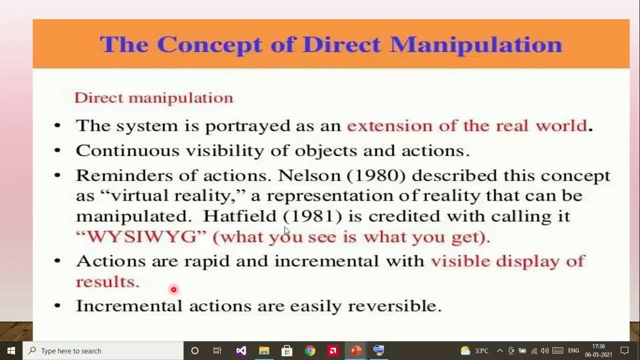 You are going to save the A particular file So that time Auditory feedback Also be possible. Sometimes you can, It in the reserves can be in a visualized manner. You don't get it as a, just like you're using smartphone. 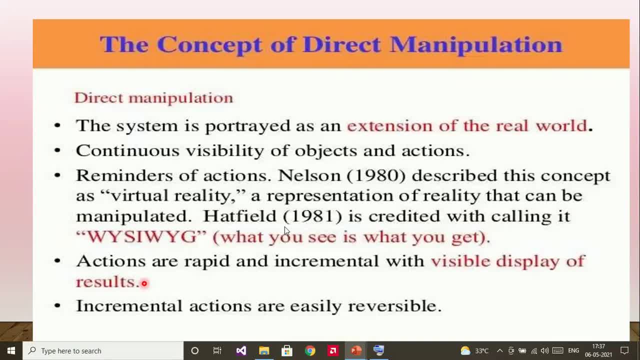 You get some feedback like that Okay Lately. when They use in the user interface we see The field as a visualized feedback or the auditory feedback is possible. the impact of the previous action is quickly seen and evolution of task is continuous and effortless. the next point is incremental. 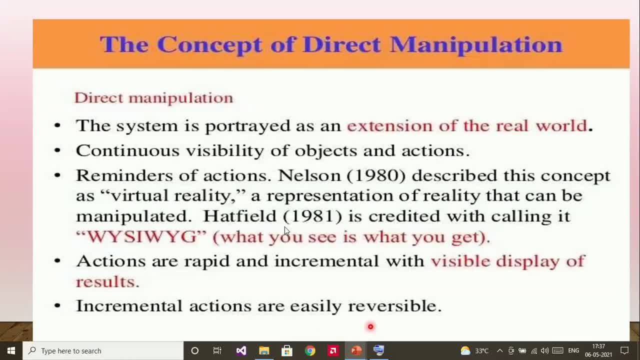 actions and are easily reversible. so, finally, whatever the actions, whatever you have performed, if you discover it as incorrect or it is not desired, okay, then you can easily undo it. so that thing is also will be done. maybe you say, when you are developing any ppt, for example, you 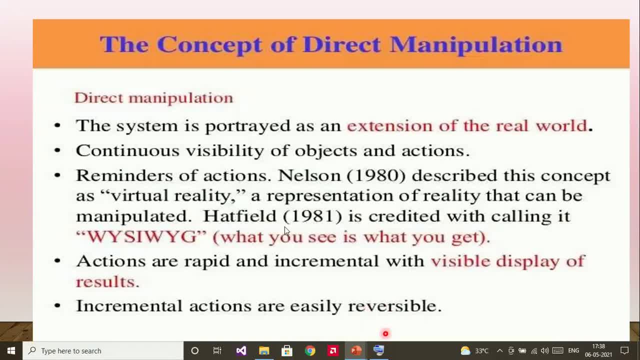 you feel that ppt is not very interesting. is it so that time you can undo your actions? whatever the actions you have performed, you can do it, or reversible. reversible actions are possible here. so this is all the characteristics of direct manipulation. so let me show an example for direct manipulation. 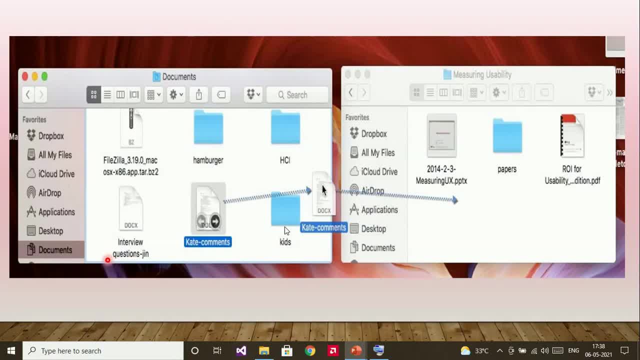 see, here you have a window that shows documents, okay, and it has some files. it has file file zilla, hamburger, etc. see, i interview kate comments like this: he had, it has got some certain files, okay, now the user interacts. he wants to just drag and drop this particular file- that is kate comments- to another. 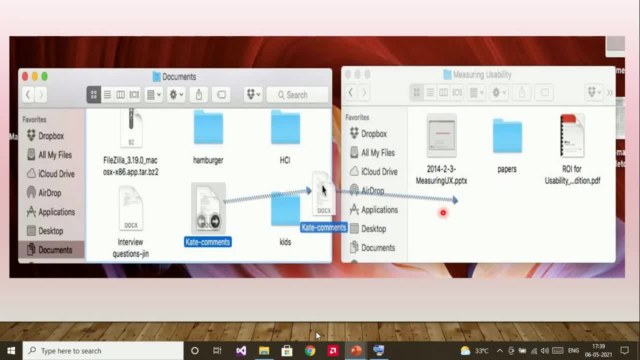 another folder. okay, so he can do it very easily, is it? he can do that, this task, very easily. so, uh, the first characteristics: the system is portrayed as an extension of real world. that means dragging certain object. here the dragging certain object is done and it portrays the real. 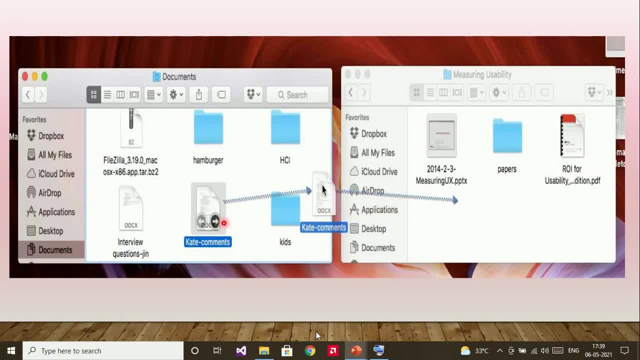 world see this first characteristics is seen here and the next characteristics is uh, continuous visibility of the objects and actions. so, whatever the actions you perform- maybe you are dragging certain uh file here- okay, that is seen continuously. here is it: visibility of the object and actions are continuous. and next point is actions are rapid and incremental. 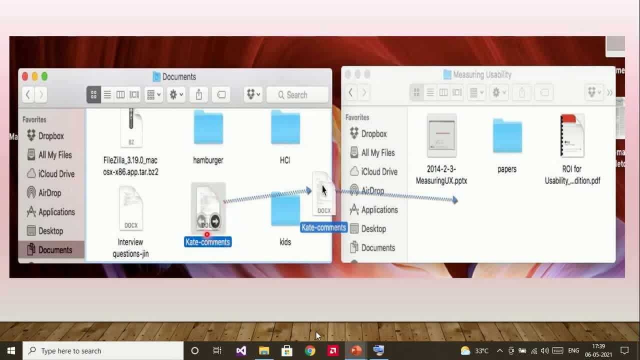 with visible display of result. so as soon as your task is being completed it will be visualized in the next folder here. is it directly, the result is visible directly on the screen and incremental actions are also possible, or is it? incremental actions are easily reversible, so that means suppose if you have done, you have dragged this particular document and you 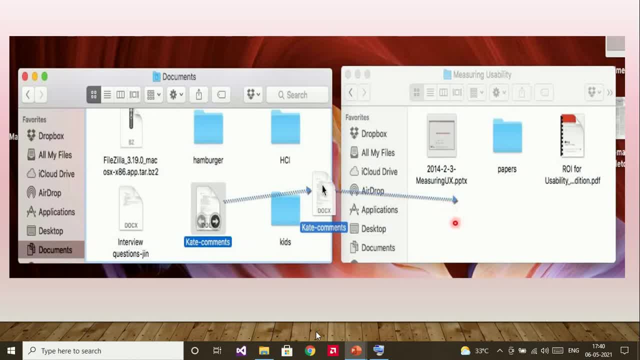 have placed it in another folder. okay, and uh, suppose here the k8 comments. you have placed it already in the uh folder here. that is named it as i'm named it as measuring usability. okay, so this uh task, whatever you have performed now, can be reversed. okay, that means you can. 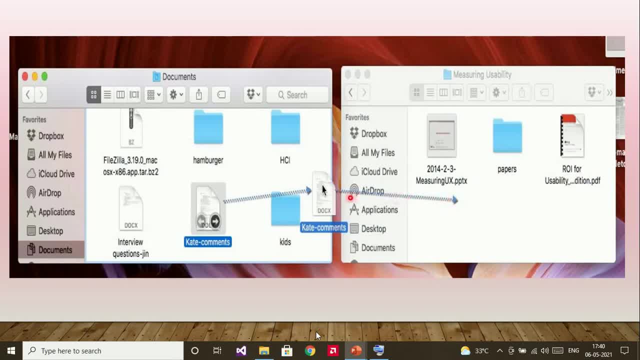 undo it, undo the operation and you can keep back the same five kate comments on the uh previous location. so this is an example here for direct manipulation.